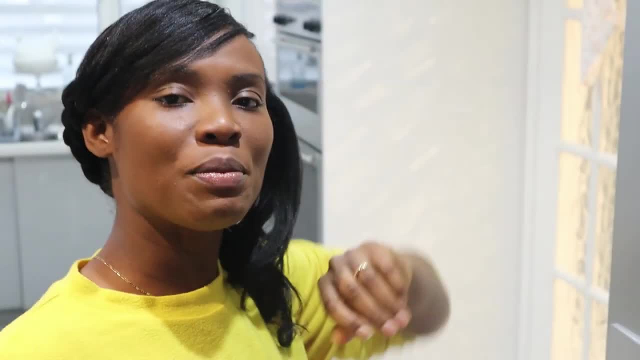 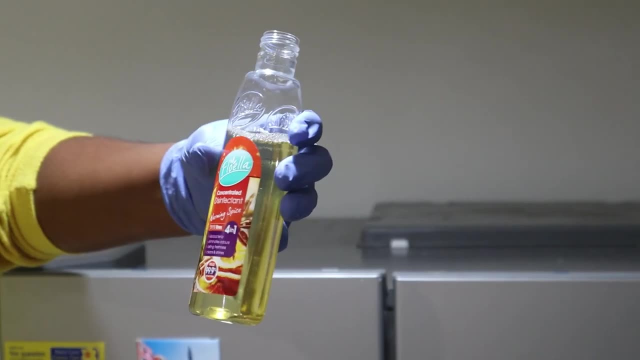 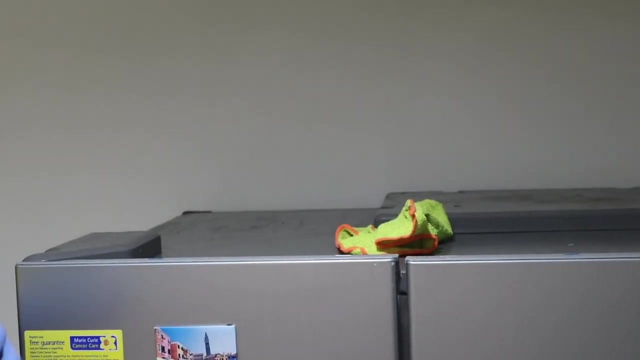 minimalist and love them. come along with me. and exactly what to do. right, and I'm just gonna go in with my disinfectant arm for Hila. you can get this anywhere, guys, you don't have to use it. just a bit of soap and water is good enough. but 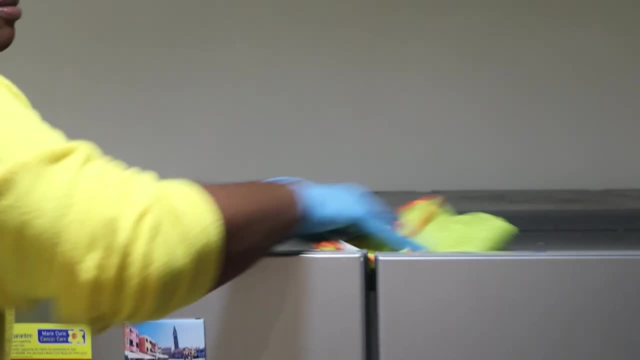 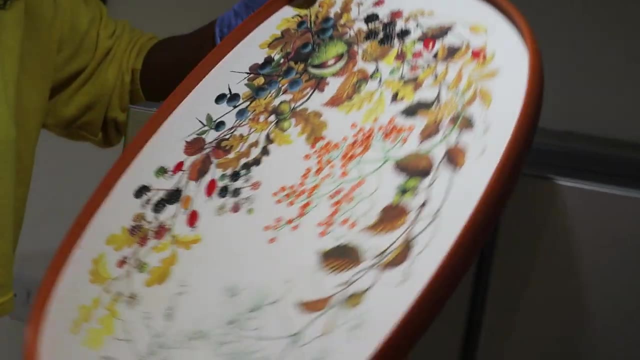 just want to give it a nice fresh smell. right, I'm just gonna use this tray that I've got here sitting in my cupboard for a while. it's very old-fashioned, but I'm gonna use it today. reason being: I want to show you how to use it today. I'm going to show you how to use it today. 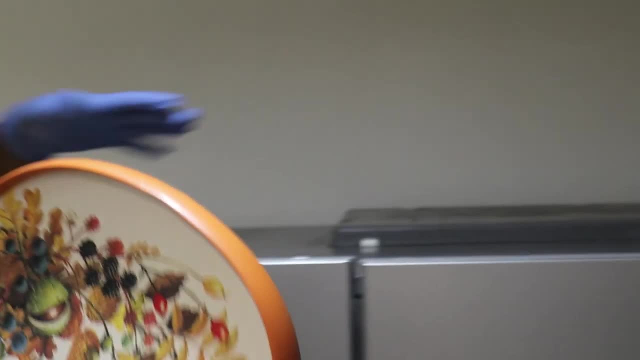 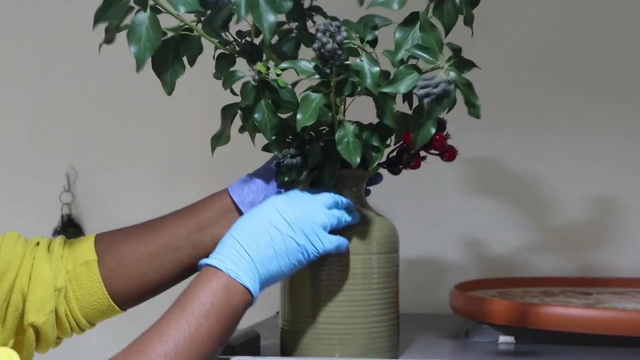 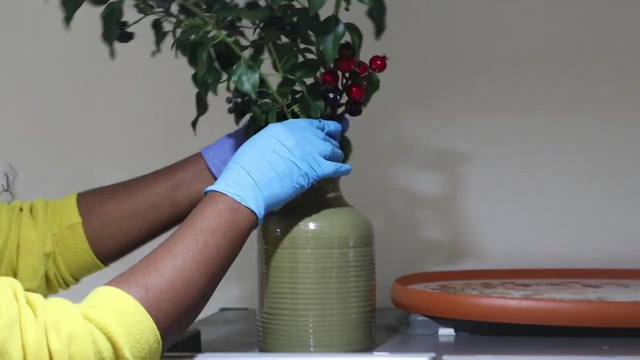 want to put the plant here, and top of the fridge is quite warm, so this is gonna work perfectly for me, okay, so I'm just gonna place my little job. guys, you can get this job from Primark. it's so, so beautiful and I just take this beautiful. 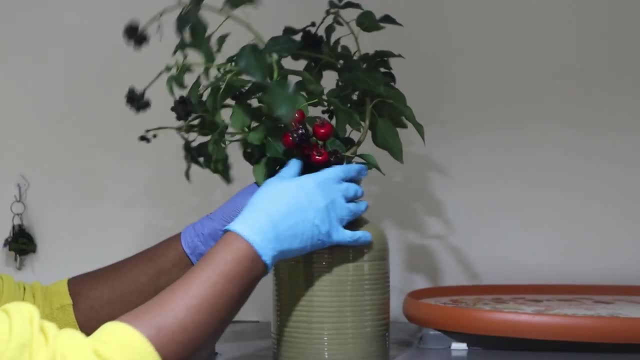 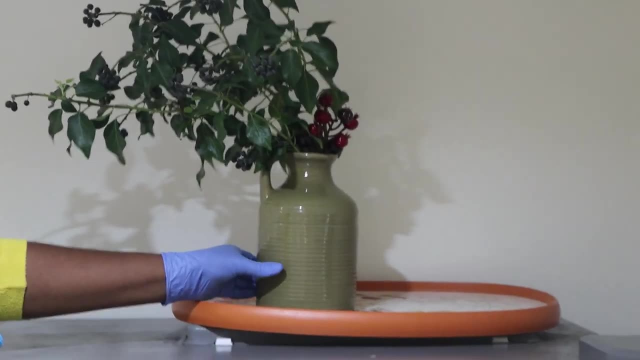 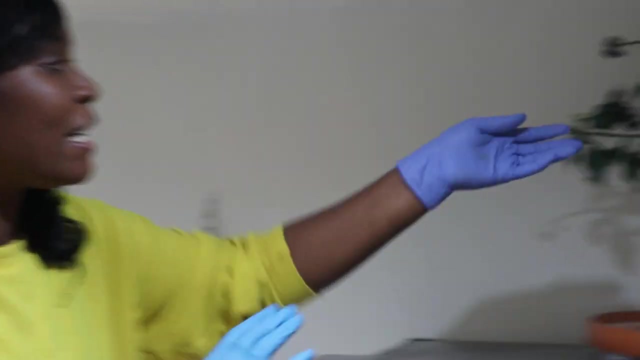 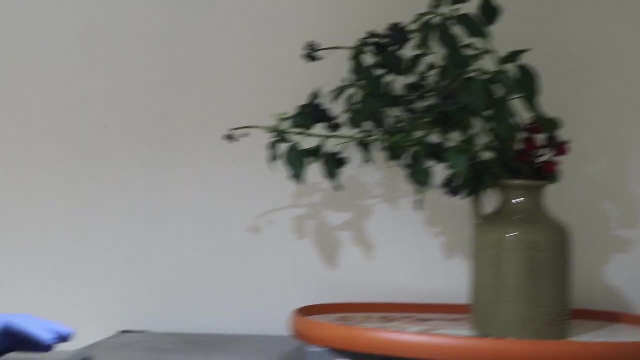 green plant that I've actually picked from outside right giving me a bit of flow, so I'm gonna just stick it here. yeah, so you can get this guys from. you can just pick this from outside, and I love the way how it has the little grapes on here. it's beautiful, love it. 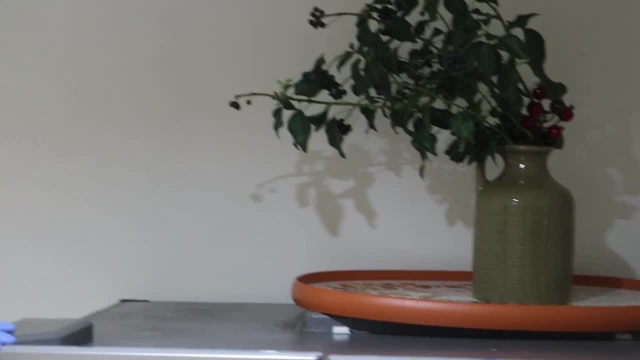 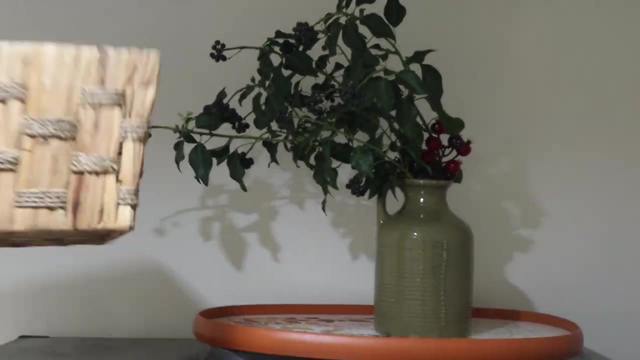 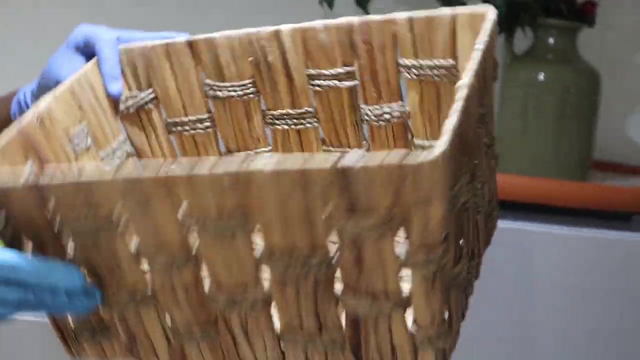 that way. right now, the next thing that I found that you can actually do is, if you're really short for space, you can get these lovely basket again from Primark guys, and it comes with a set of two, so I'm gonna be just using one here for now. 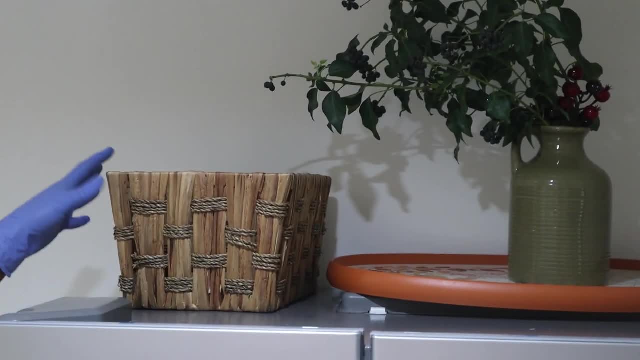 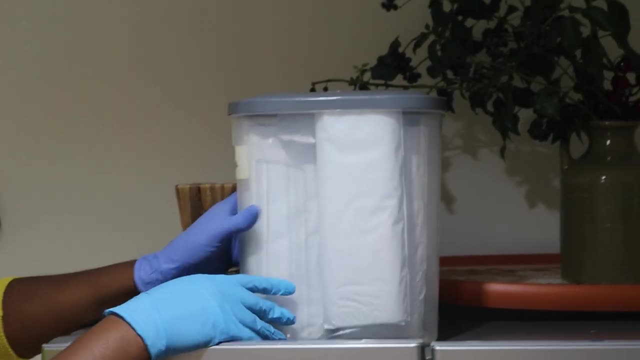 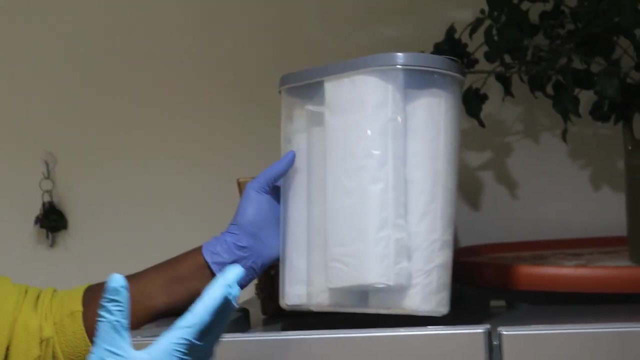 because you don't want too much on top of your refrigerator, okay, and if you are really tight for cupboard space, this is how you can actually organize your cereals. so, instead of putting them in plastic bags and packing them up in boxes, you can get these containers, guys, from really, really cheap sources, and 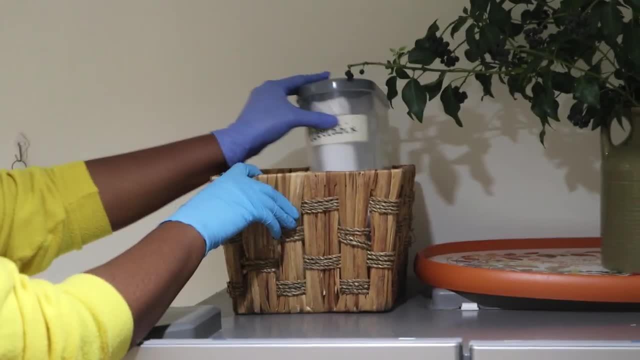 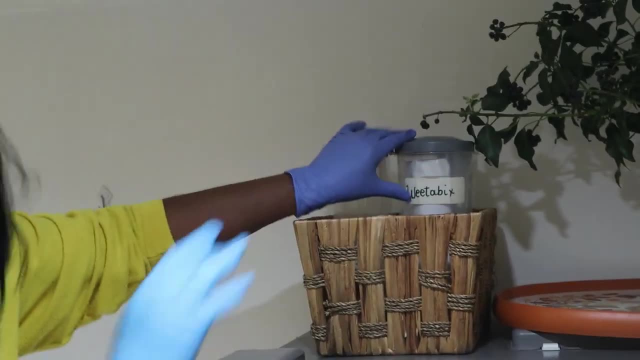 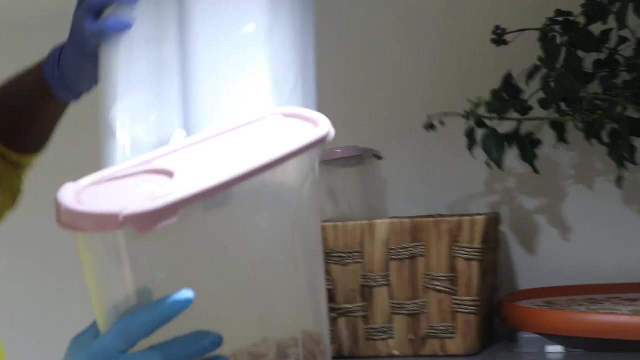 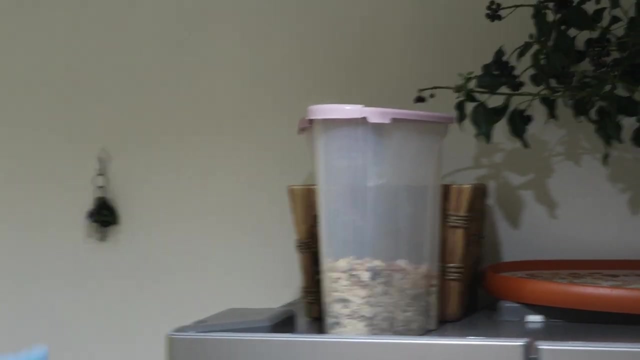 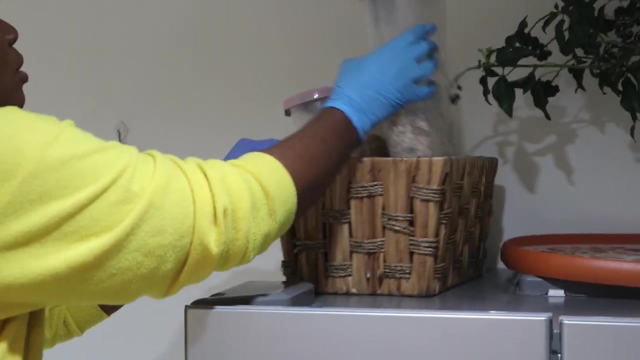 use for your cereal and you put the cereal in this one again as much as you can fit, okay? oh, this one is quite chunky, so I might find somewhere else to put it, just to accommodate more what I'm doing here. I'm doing here, I'm just showing you guys an idea. 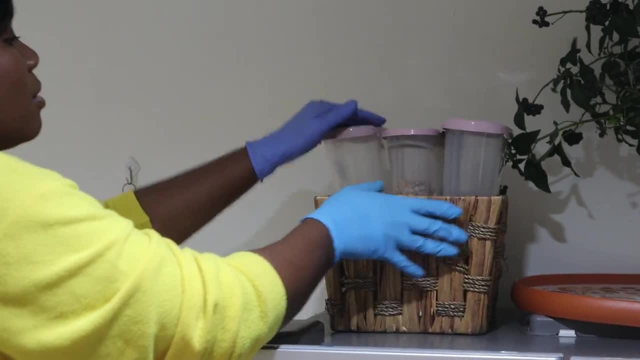 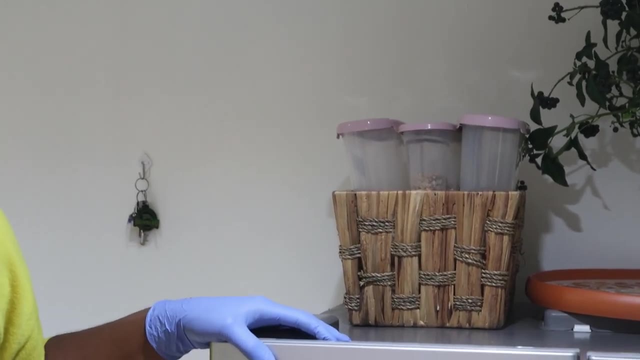 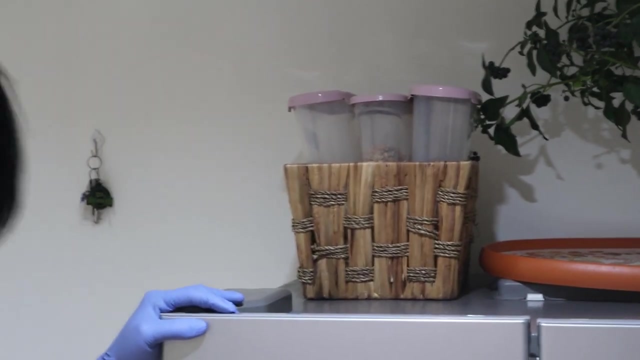 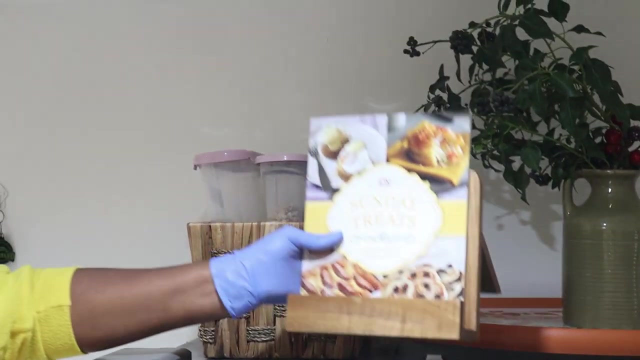 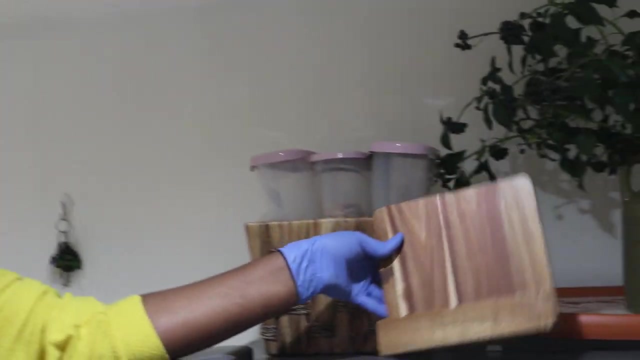 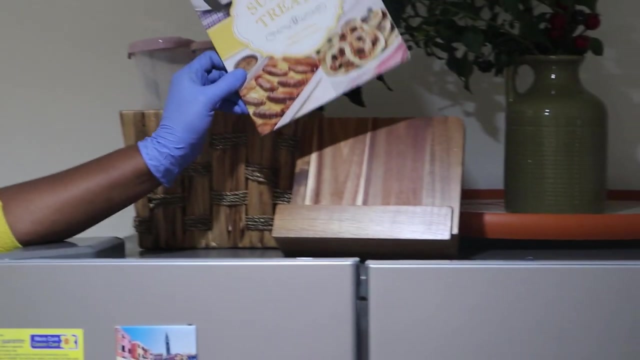 okay. so you've got that your cereal, okay, and the next thing that you want to do is: it's not too much stuff. then this is a little tray that we have, or you can put a book on it. you can put one of these kitchen cookbooks on top here. all right, okay, and I'm just gonna use. 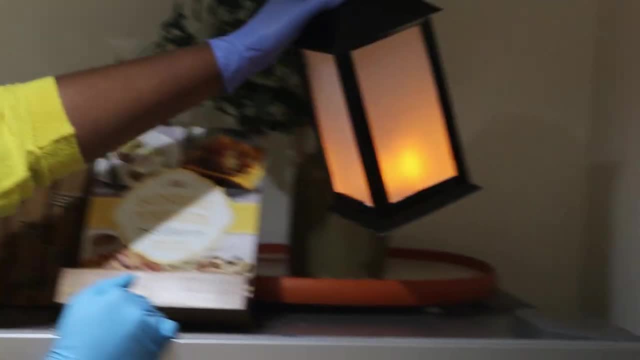 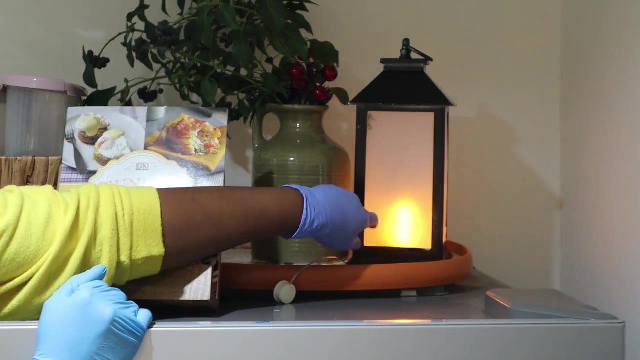 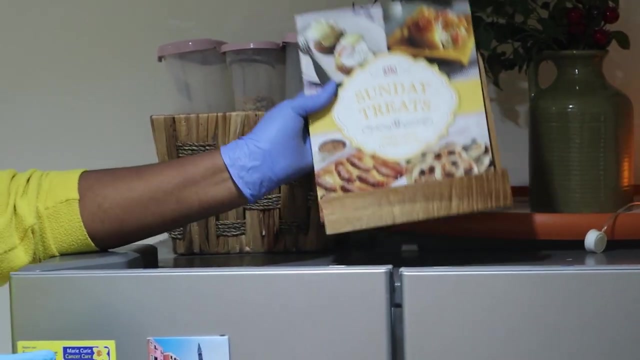 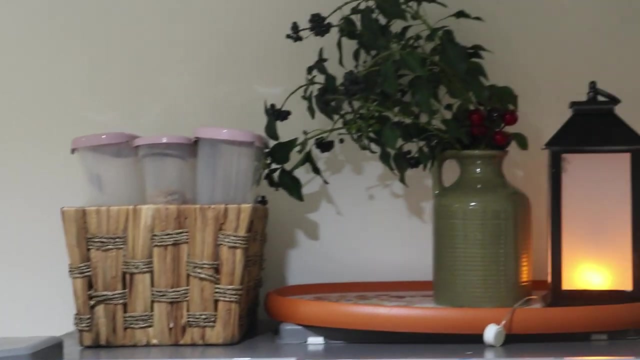 this little lantern here as a decorative piece I'm gonna put over here of all these pieces. okay, this is just an option for me. i think i'm going to remove this and put it at my face. lint, so i'll put it on the counter for this, but you 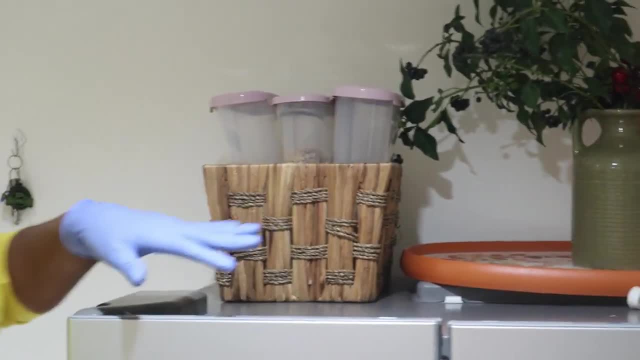 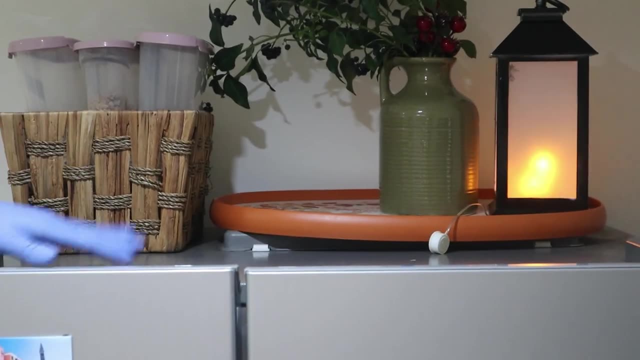 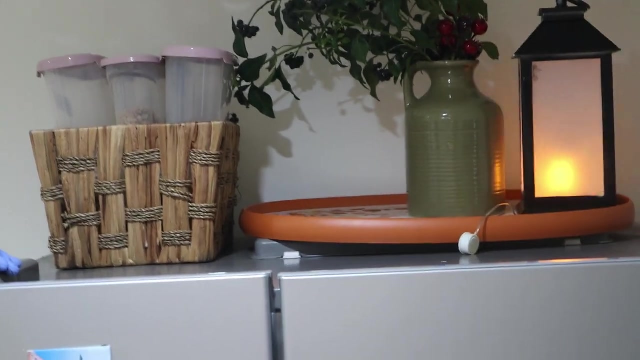 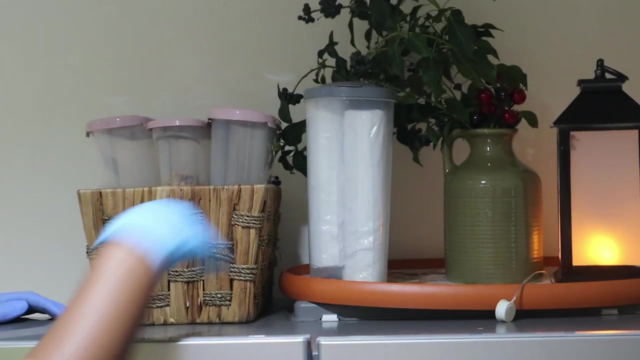 can also put your little stand up here, right? so there is still a lot of more spaces here that you could actually put more stuff. okay, but you don't want it to be too overcrowded. So I mean, because this is a bit bigger, it's not fitting in there. you can actually style. 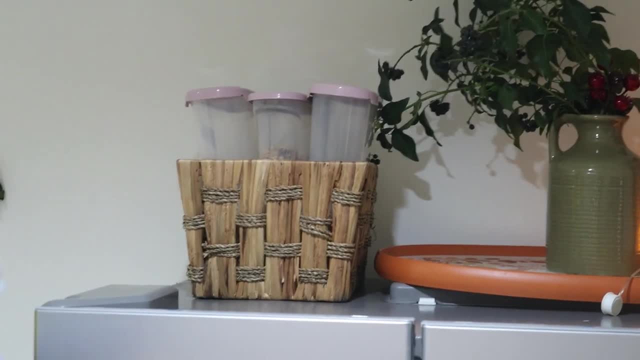 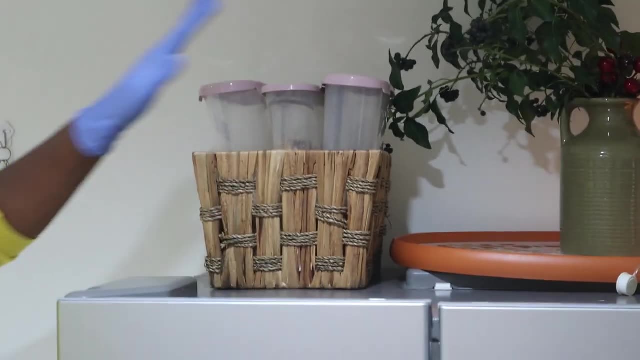 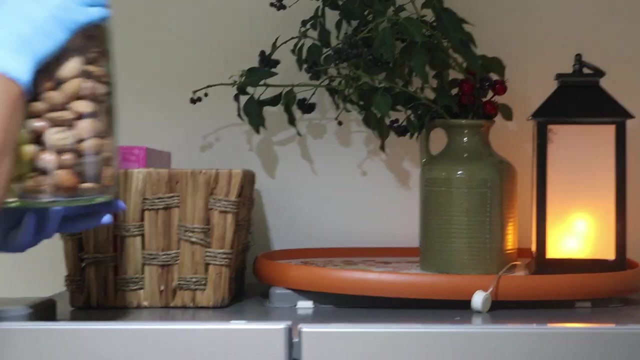 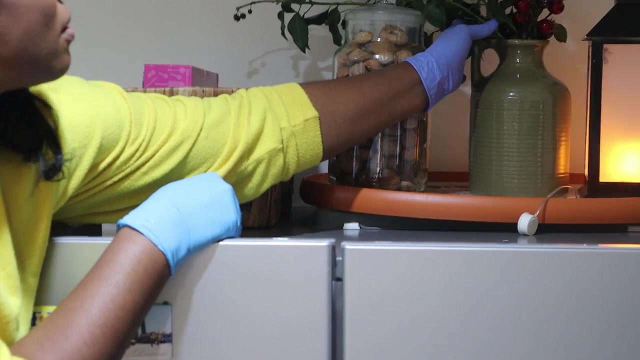 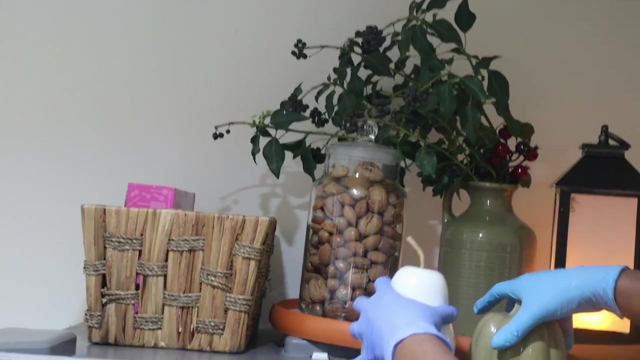 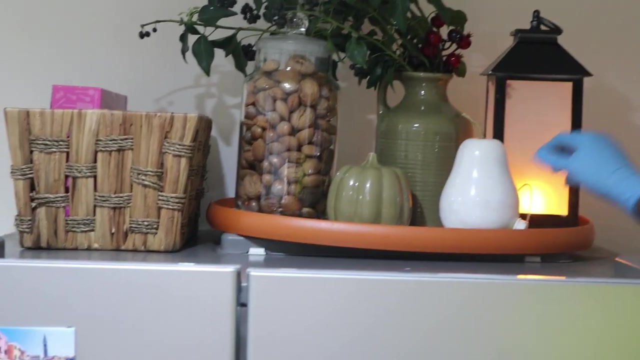 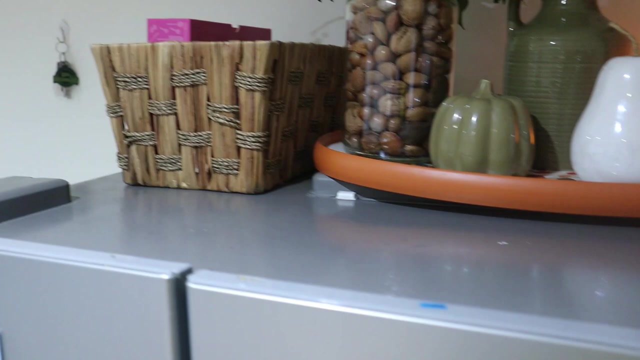 it like that For me. if you want to keep your cereals in here, that's fine. So I keep my cookbook in here, guys, okay, All right. So that's the ending, and there is still a lot more space on top of my refrigerator. 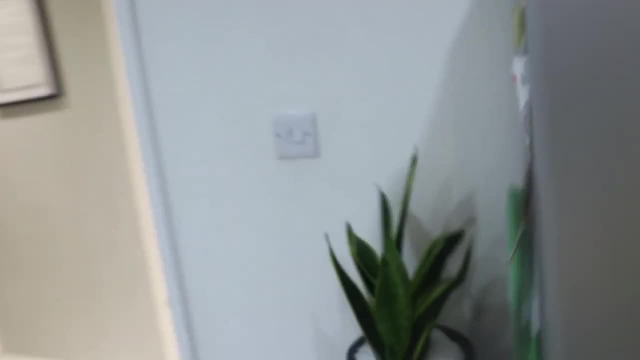 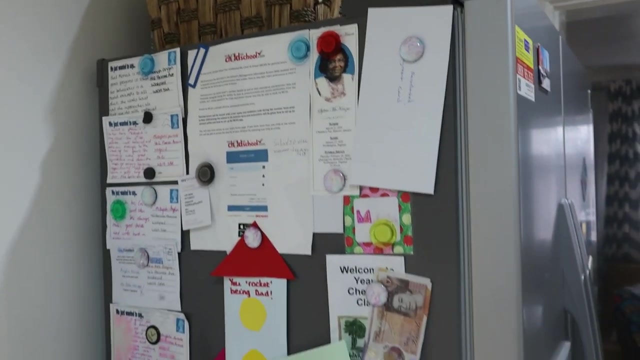 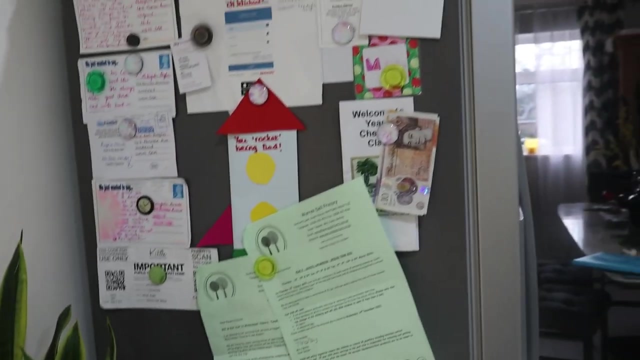 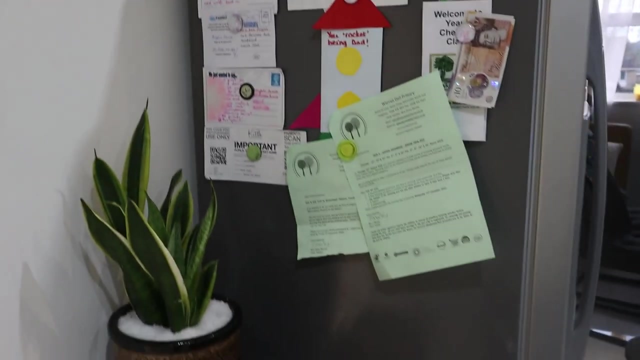 guys Coming down. I think lots of households tend to have papers on the refrigerator sticking up just to remind you to do stuff, or you know, and I felt deeply that it's not really looking all that stunning. It takes away a lot of space. 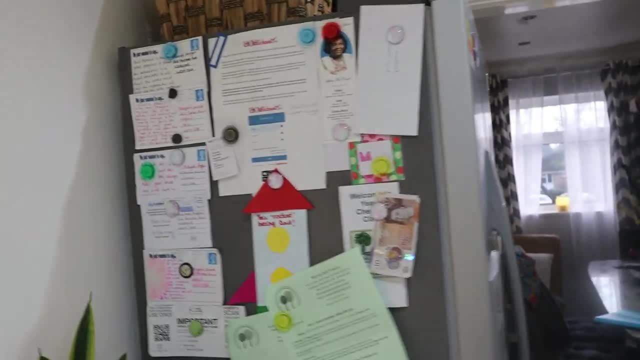 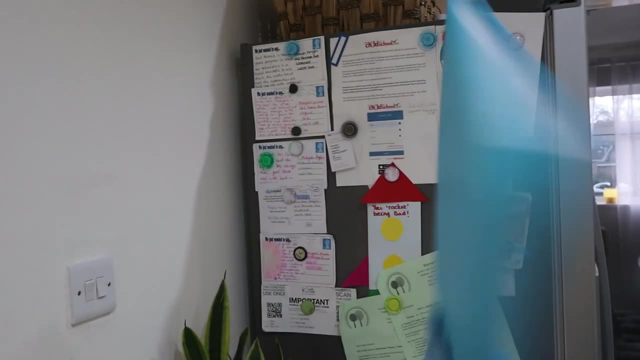 It takes away the glam. it looks a little bit cluttery. So I came up with a little idea and just stay tuned as I show you my idea. So right guys. so I'm going to be using just one of this folder here, with different sections. 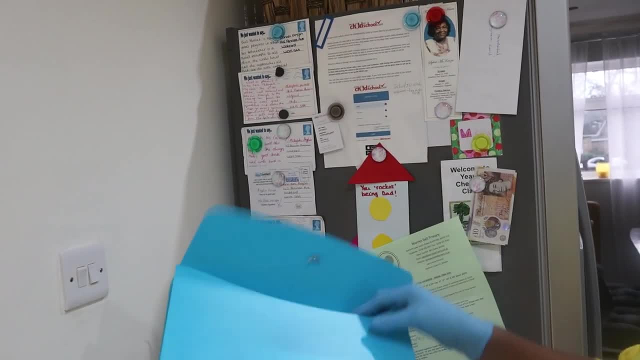 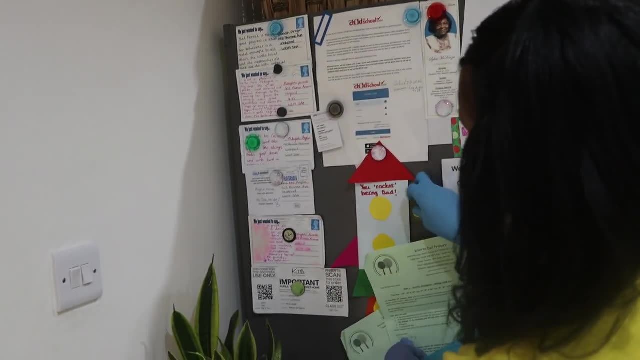 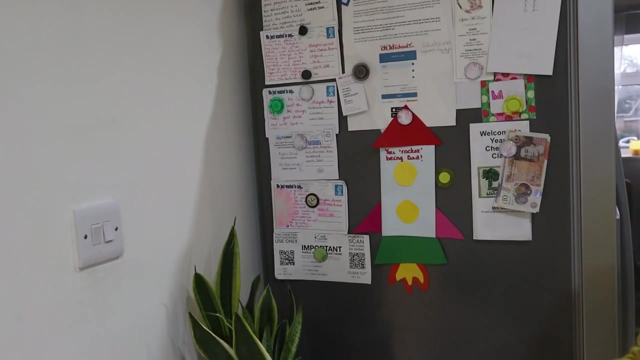 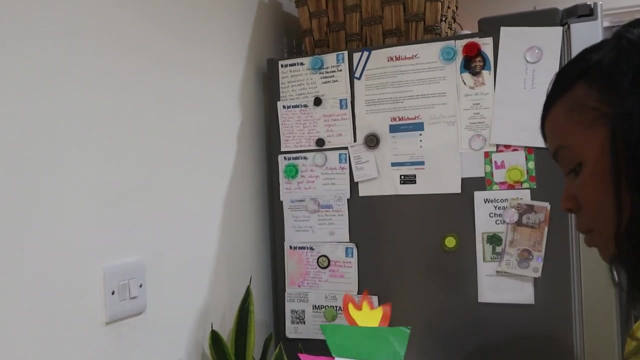 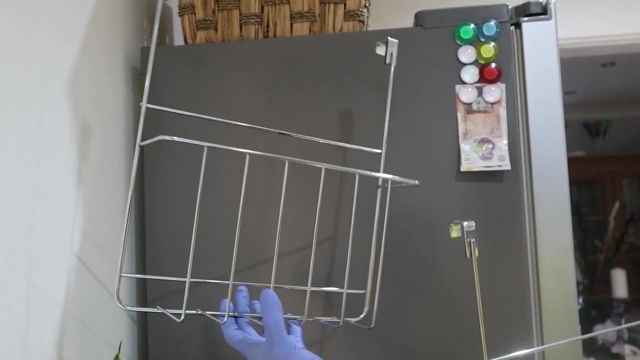 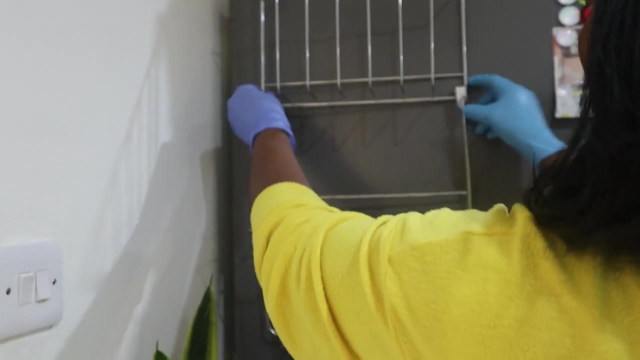 okay, And so I felt like All these documents can be fitted in here. Okay, guys, so this is actually some pot cover holder that I'm going to be using here as well. I've got them for a long, long time, which I've thrifted. 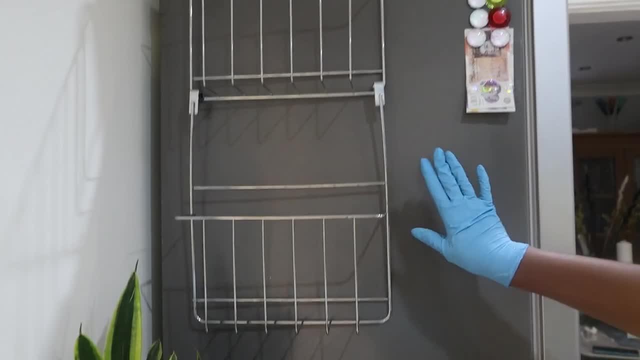 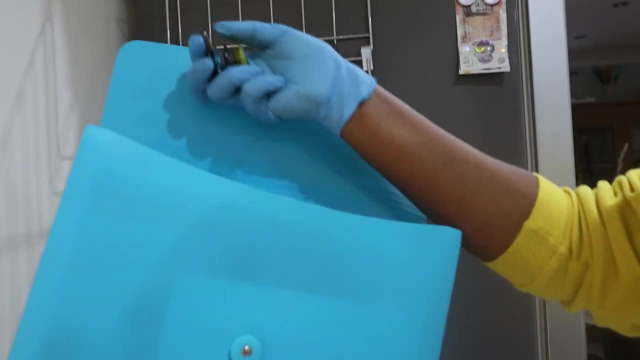 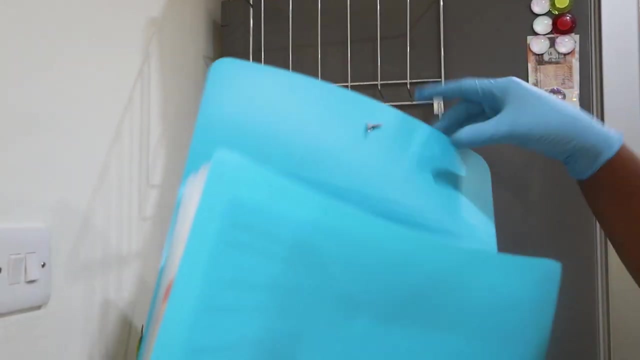 Right. So all the papers, All the papers that was here, I've actually put them inside this little folder here, and I've got the remaining magnets for the fridge. I've dropped them in here. So if I need, I can just go in here and it's all organized and ready to be used. 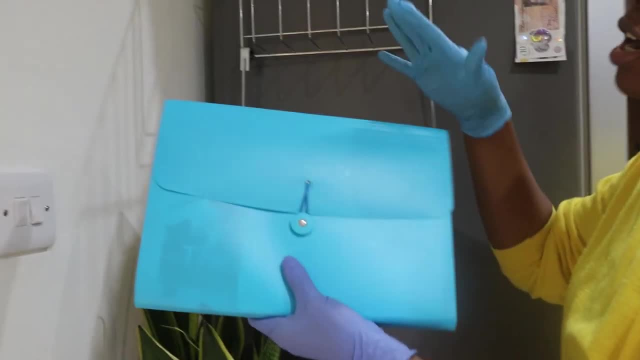 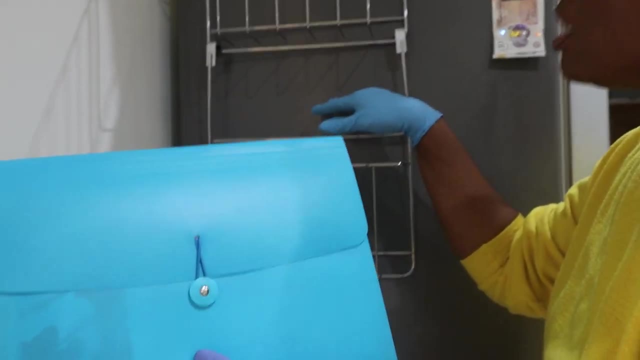 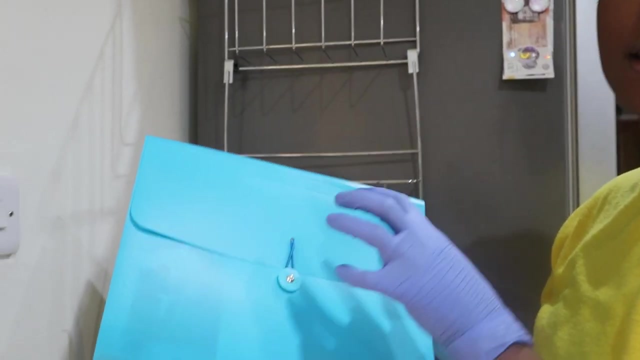 But for future reference, I believe I will get a gray, a gray folder, So instead of a blue, you could actually go for a gray or a white- So it's, you know it's flow- or a brown. So as soon as I go to the town, I'm going to be getting a color that will coordinate. 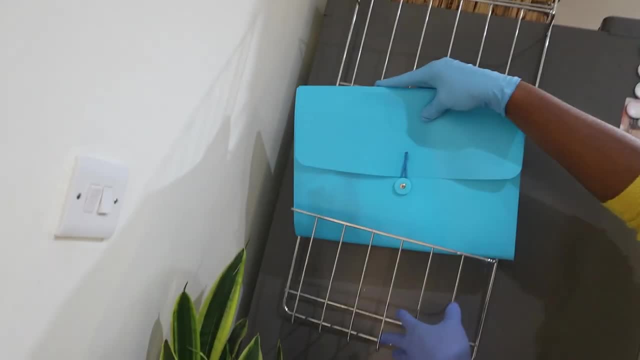 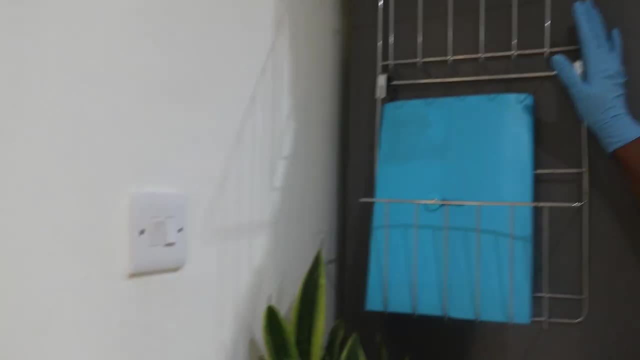 with my kitchen. So yes, guys, so you can actually put this folder in here. it doesn't fit that way, it can fit this way, All right. And the rest of the remaining space- I mean, guys, you can use, you can put anything in. 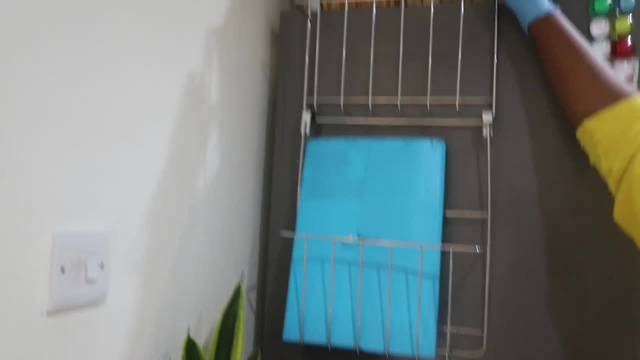 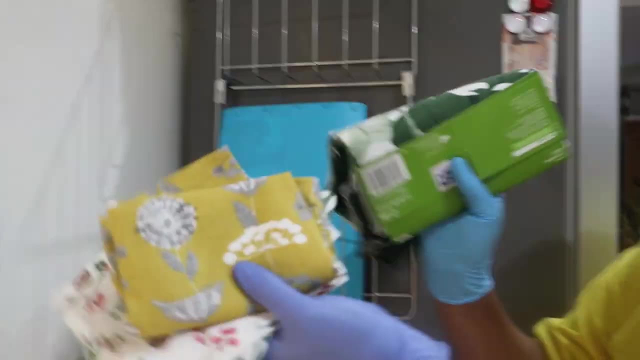 here You can put water. I mean, you don't want to put too much heavy stuff, but for example, I'm just going to show you what else you can do with the space. Okay, So the last space here: kitchen towels. 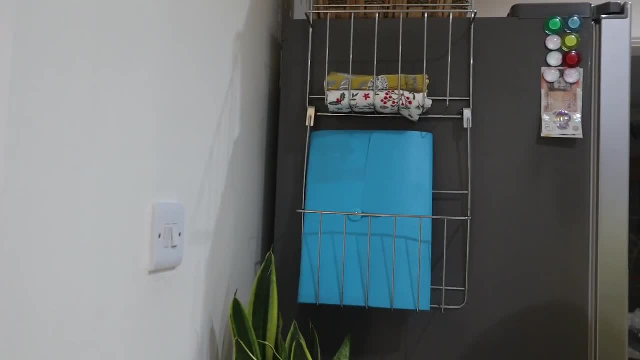 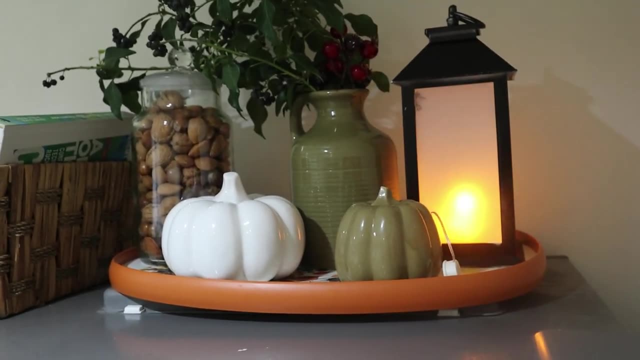 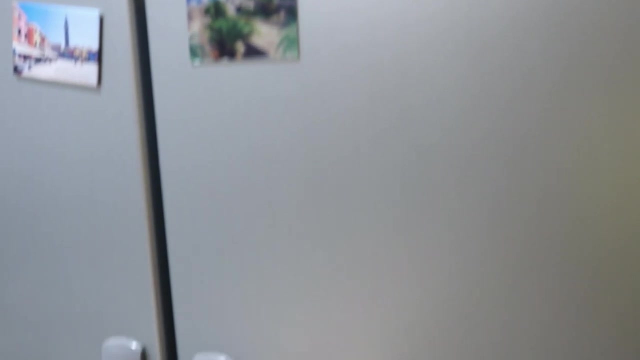 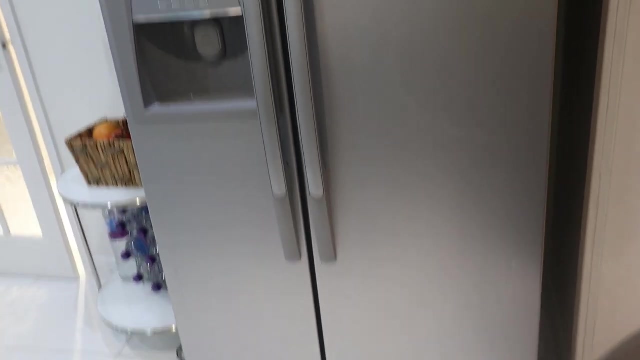 So this is a wow-wow. Okay, guys, So that's the finished look of my fridge refrigerator, the top of my refrigerator. As you can see here, this is my refrigerator, So that's the top. It looks so beautiful, All right. 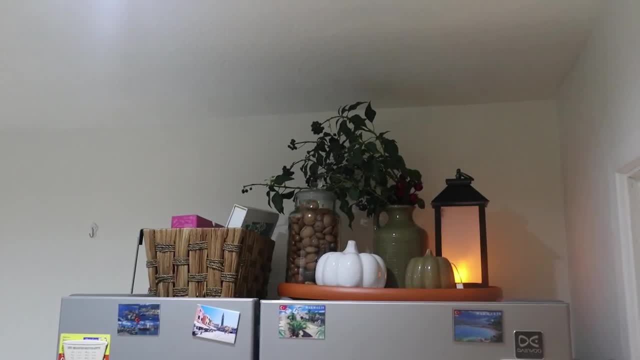 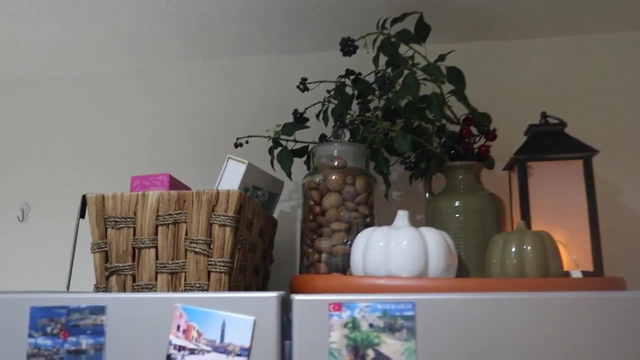 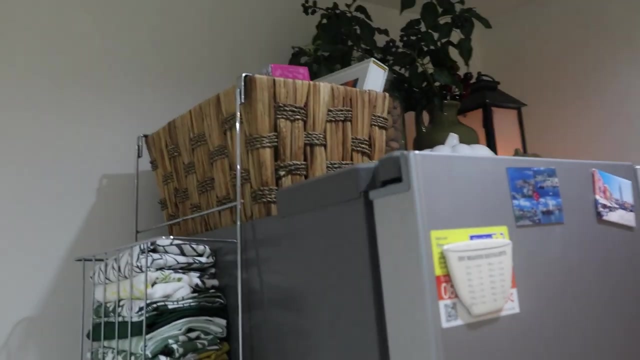 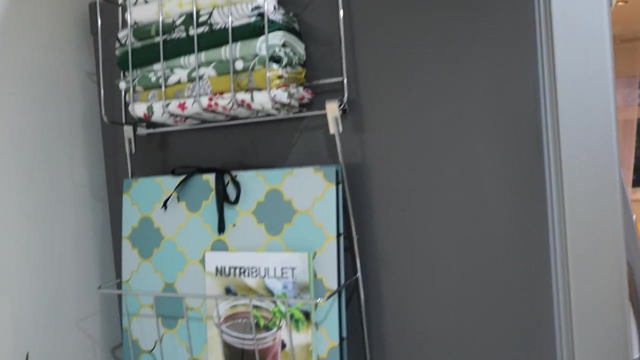 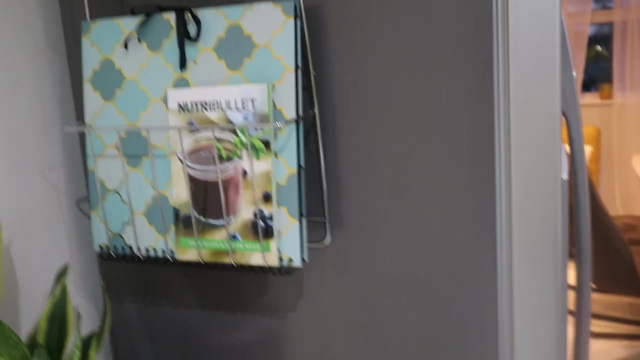 And just at the side of my refrigerator I had a lot of papers and so forth. So I took all those filing all those papers and I filed them away into this lovely book here. You can also file them away in a nice little wallet, something like this. but because the 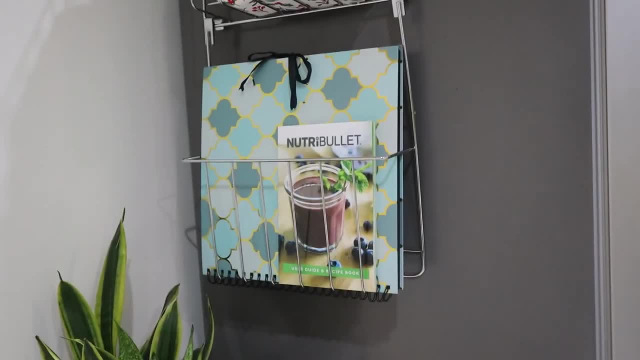 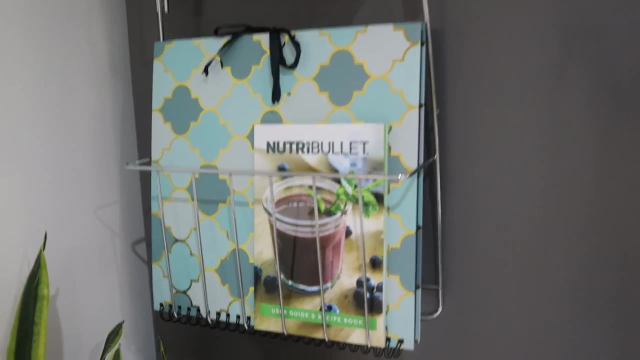 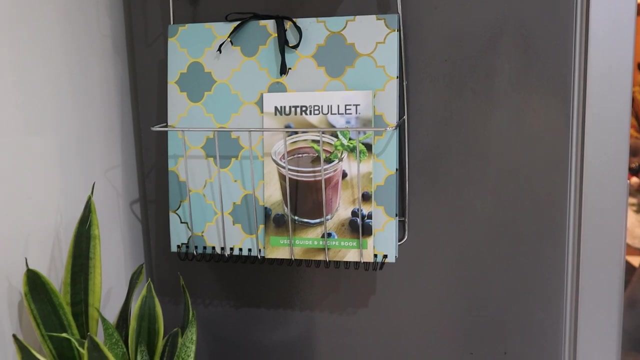 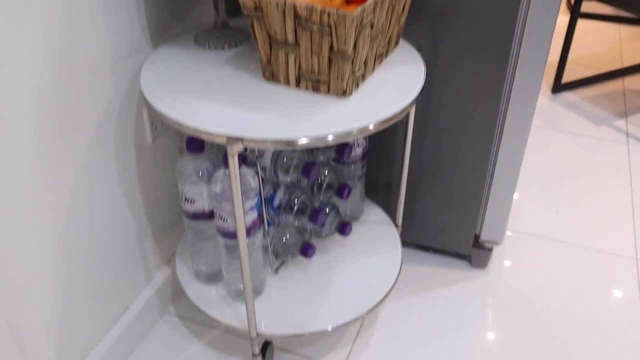 color is so blue and so bright. I actually sort of shocked my home and I found this lovely little purse book and I felt it's really slay. And yeah, And just below that I have this book, I have this wonderful, beautiful table with the wheels on it that you can actually put. 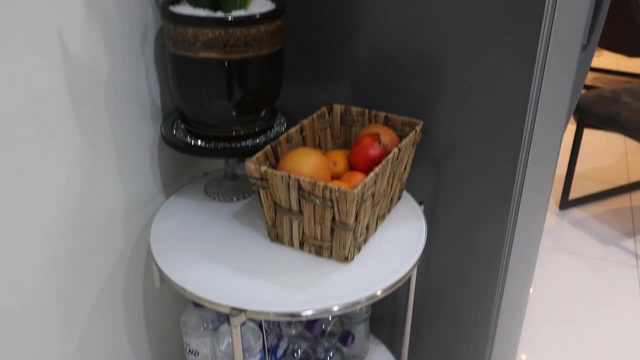 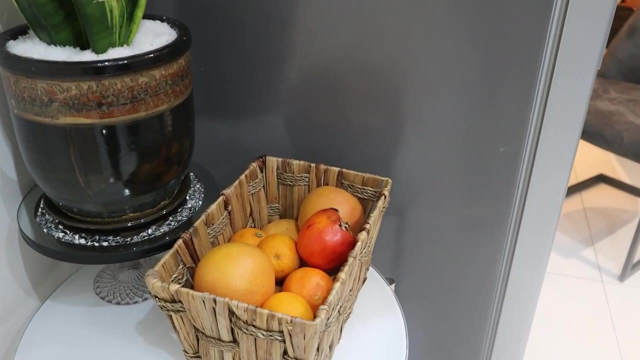 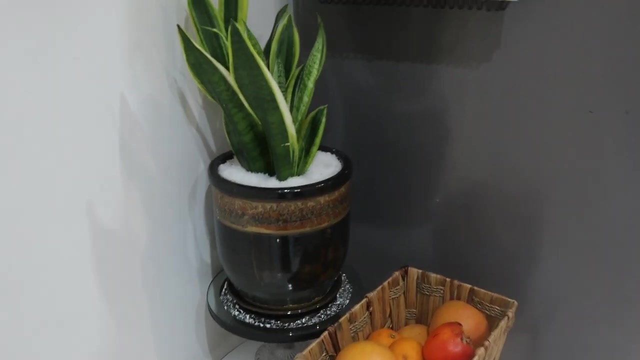 wine and so forth on. And I tend to have my foods here- grapefruits, especially where I'm sort of picky when you come onto grapefruits- Very good for your bowel and digestion as well. I have this lovely snake plant as well for years and years.